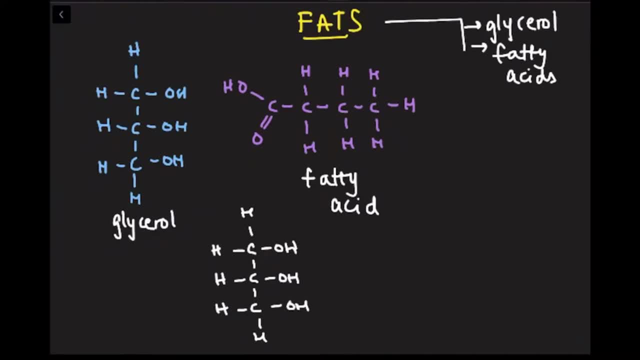 dehydration synthesis. What happens is the hydroxyl on the fatty acid and the hydroxyl on the glycerol molecule combine to form a water molecule and an extra oxygen. Now the water molecule leaves and it leaves this oxygen to bind both the molecules. So what ends up happening here is, instead of the hydroxyl, 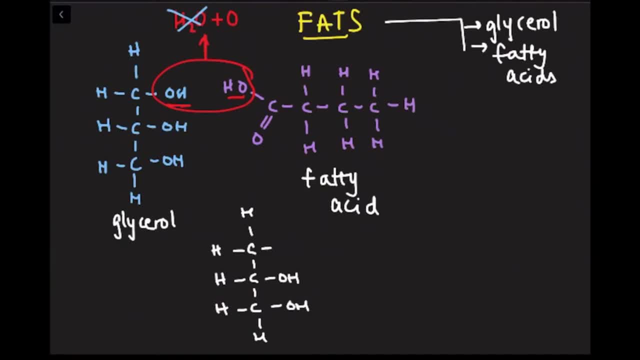 group. on the glycerol. you substitute that with the extra oxygen and you add the fatty acid to the end of that. So you add your hydrocarbon chain, and this is what that ends up looking like Now. to create a fat, you need three fatty acids to bond to each of the hydroxyls. on the glycerol. 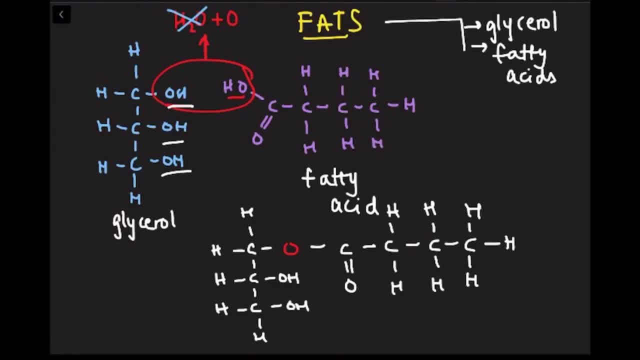 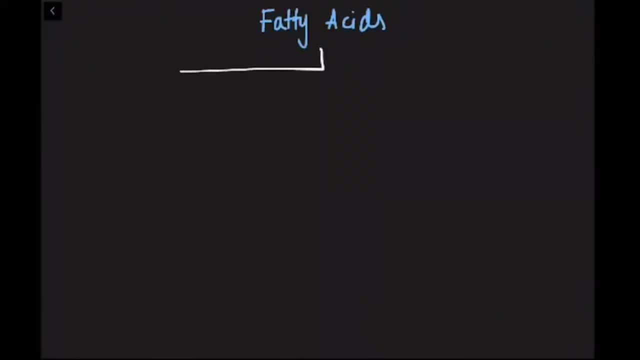 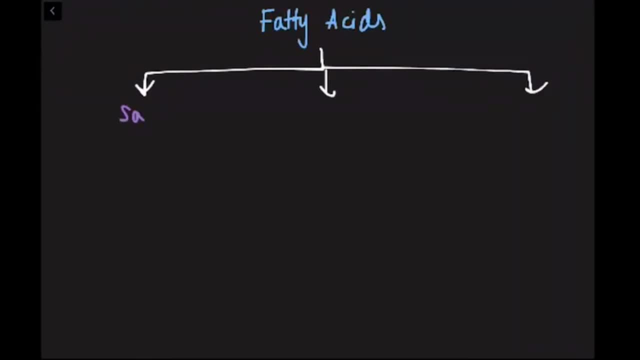 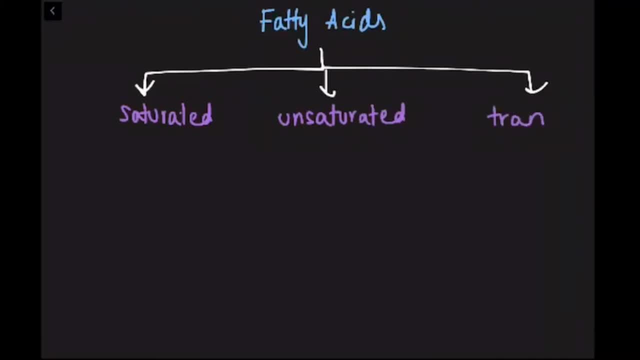 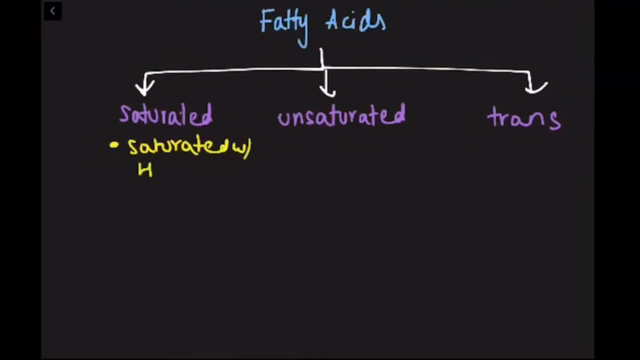 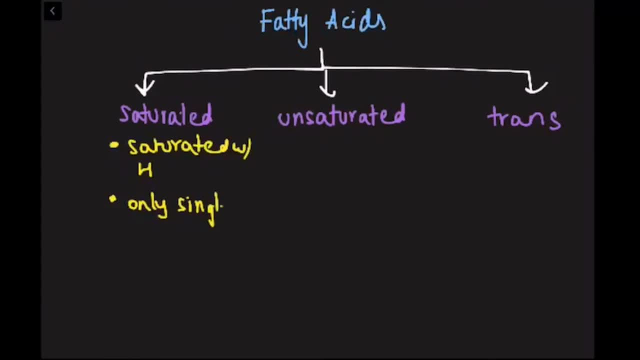 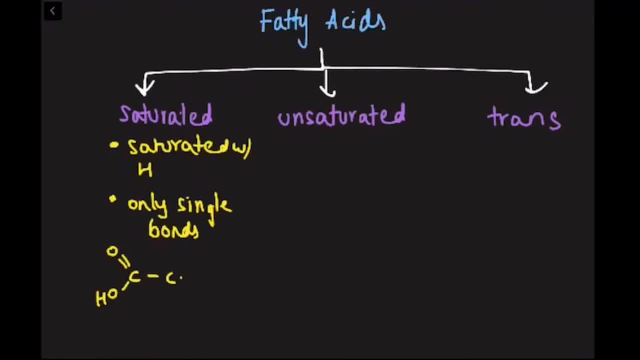 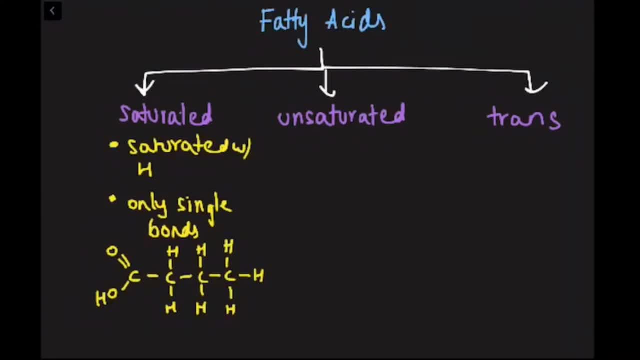 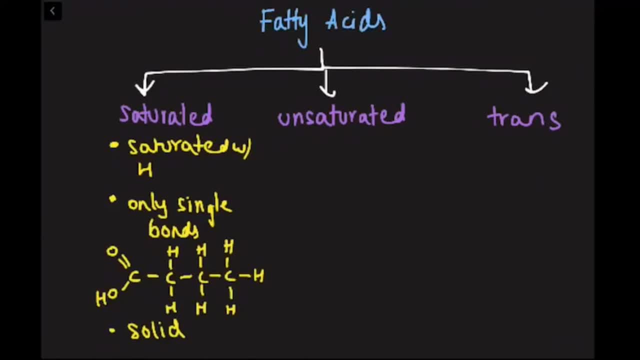 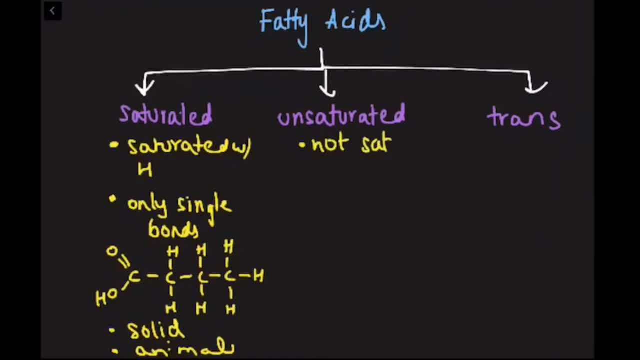 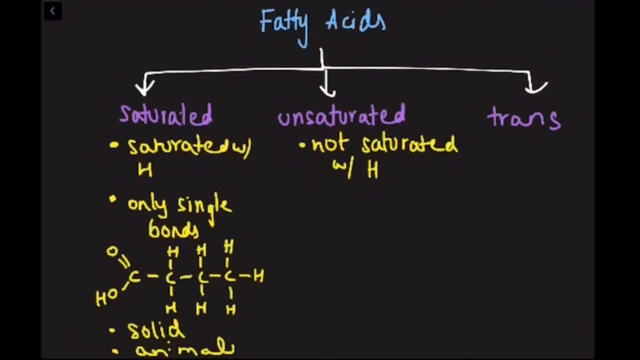 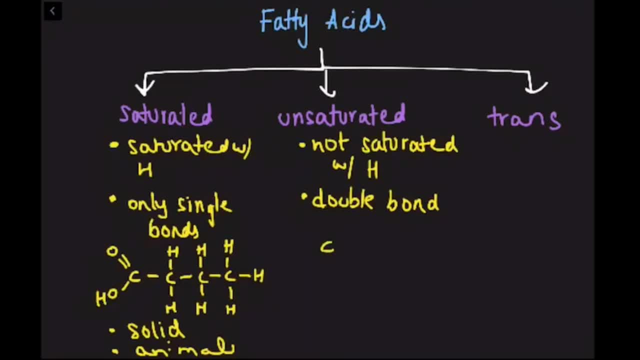 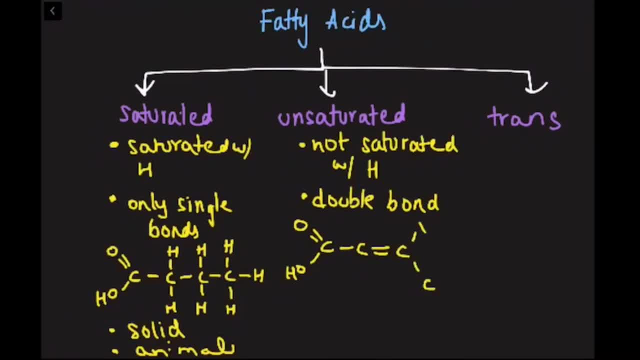 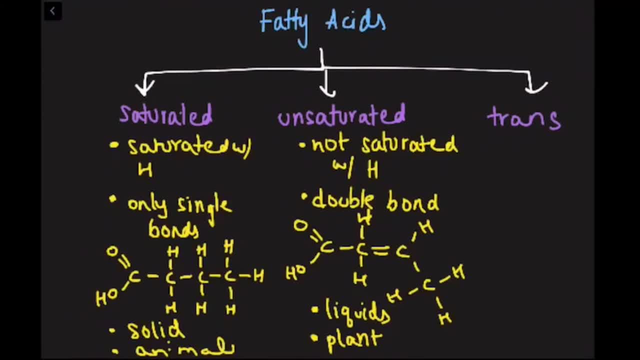 Unsaturated fatty acids, or unsaturated fats, are more healthy than saturated fats. Now, lastly, we have trans fats. These are basically unsaturated fats, like vegetable oil, that have been hydrogenated, meaning hydrogen atoms have been added to these unsaturated fats. Trans fats are even more unhealthy than saturated fats. 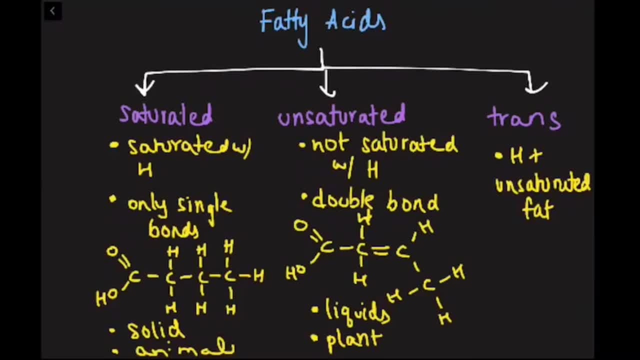 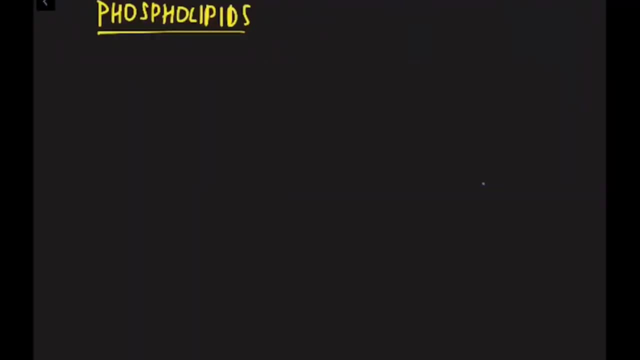 Trans fats and saturated fats can contribute to diseases like atherosclerosis. In atherosclerosis, plaque coats the insides of blood vessels and impedes blood flow, leading to heart problems, lung problems and organ failure. Next, we're going to be looking at phospholipids. 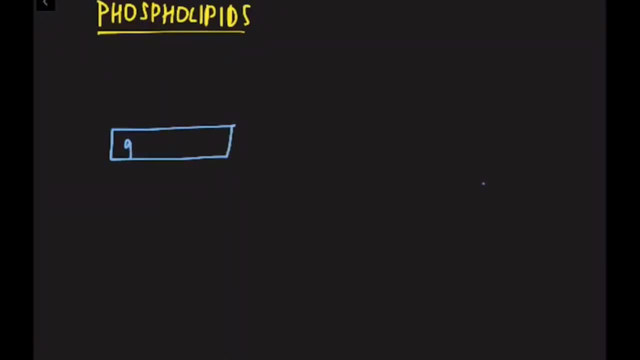 In a phospholipid, you still have your glycerol molecule, Except this time the glycerol molecule is only attached to two fatty acids. The third, hydroxyl on the glycerol, is actually bonded to a phosphate group, which is PO4 3-. 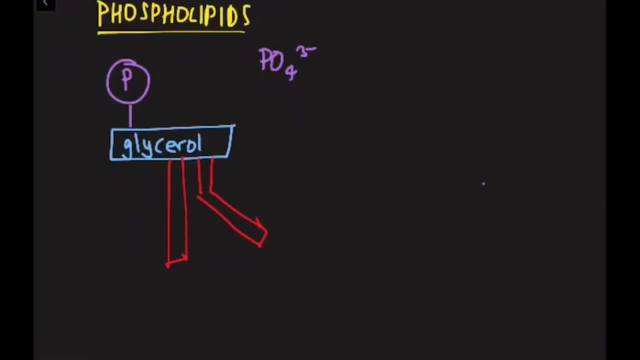 Now, the phosphate group in this molecule is polar and the hydrocarbon chains are non-polar. This means that both ends of the molecule react differently in water. While the hydrocarbon ends reject water or repel water because they're hydrophobic, the polar head, or the phosphate, has an affinity for water. 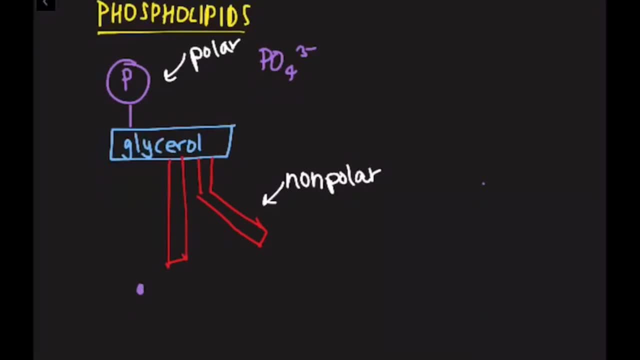 So when phospholipids are added to water, they automatically arrange themselves to form something called a bilayer, which looks like this Say: these purple dots are the polar heads. they arrange themselves on the outsides because they like water. Meanwhile, the yellow lines, which are fatty acids, are non-polar. 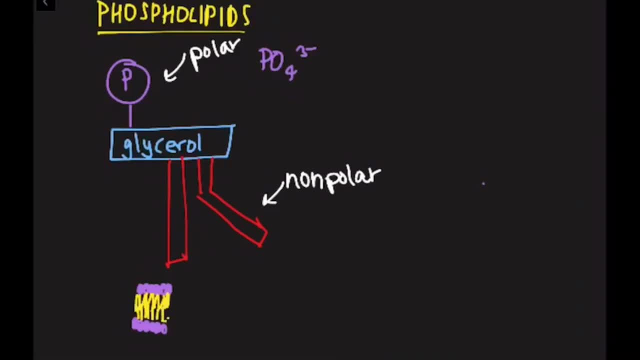 This means that they're hydrophobic. This is called a bilayer, because you have two layers of phospholipids. Our cell membranes are made up of phospholipids. Because our body is mostly water, the phospholipids form this same bilayer around our cells. 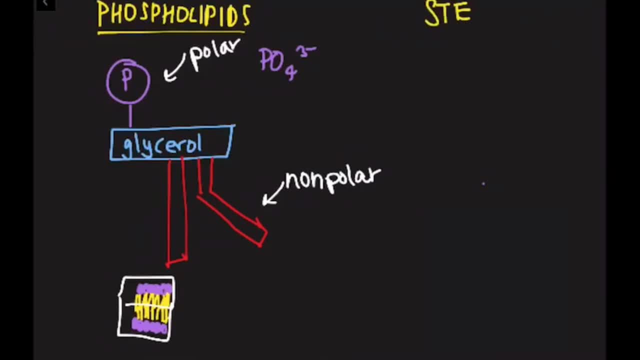 Lastly, let's look at steroids: Steroids, Steroids, Steroids, Steroids. Not really much you need to know about steroids. All you need to know is their structure. Steroids are composed of carbon rings, Which looks like this: 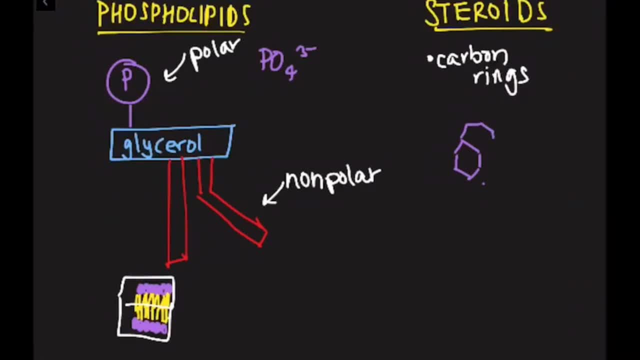 Again, there's not really much you need to know. You just need to know how to identify steroids when you're given a molecule and they just look like rings. Now, different chemical groups are attached to steroids and that's what makes each steroid different.